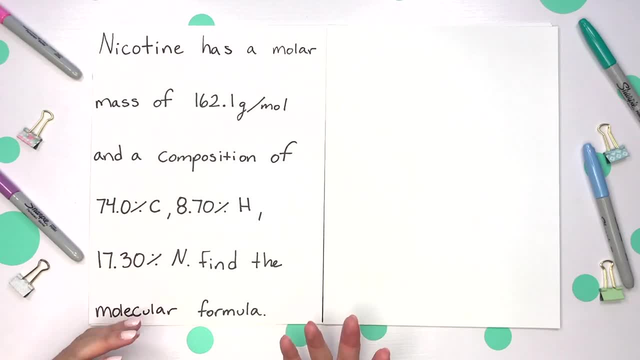 formula, you first have to figure out what your empirical formula is. So our first step is to change our percentage to grams. To do so, note that if we were to add up all of these percentages, we would have to add up the molecular formula, So we would have to. add up the molecular formula To do so. note that if we were to add up all of these percentages, it would be out of 100%. So because it's out of 100%, there is no need to multiply or convert anything. You are literally changing your percentage to grams. These will be our new. 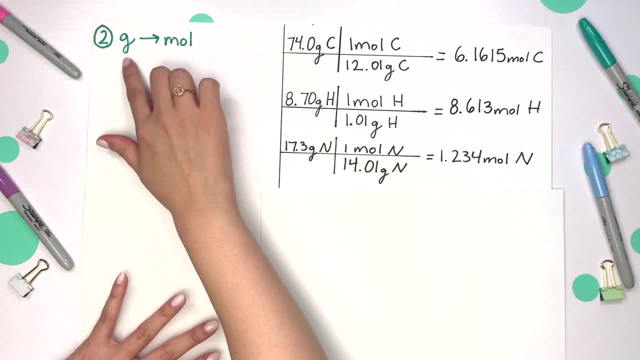 values that we'll use in the next step. Step two is to convert your grams that we found in our previous step to moles. When converting to grams to moles, we use molar mass of each element to get to moles. So in our case we'll have the 74.0%. 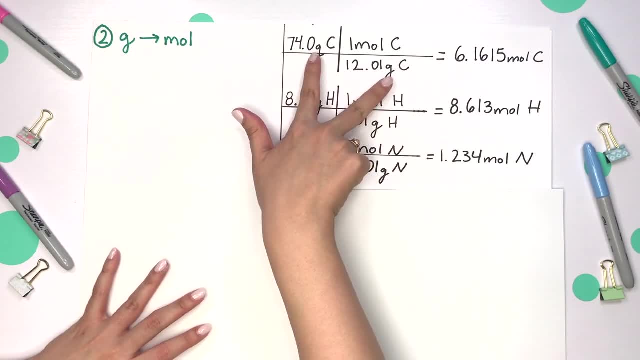 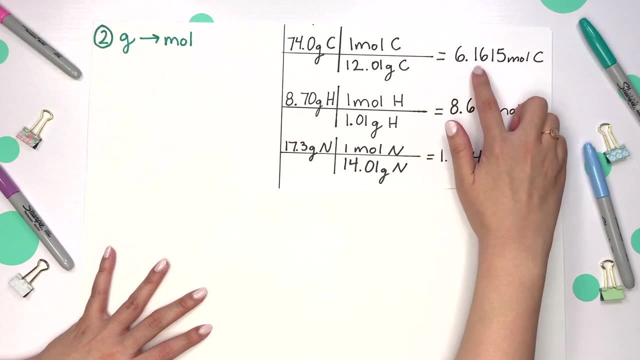 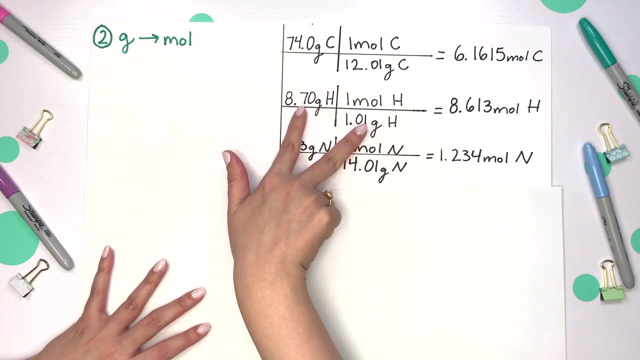 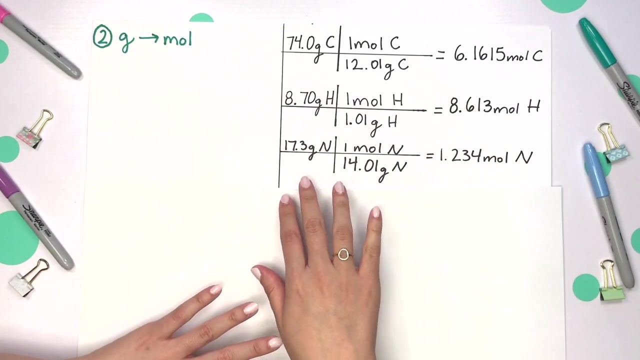 We'll do the same thing for hydrogen, except aligning hydrogen's molar mass on the bottom, And then we'll divide and you get 8.613 moles of hydrogen. And lastly, we'll do the same exact thing for nitrogen, except nitrogen's molar mass is 14.01%. 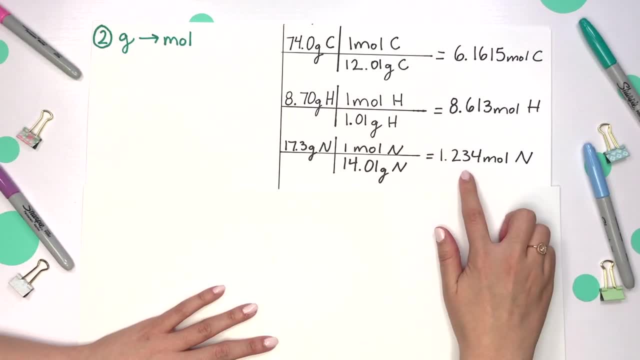 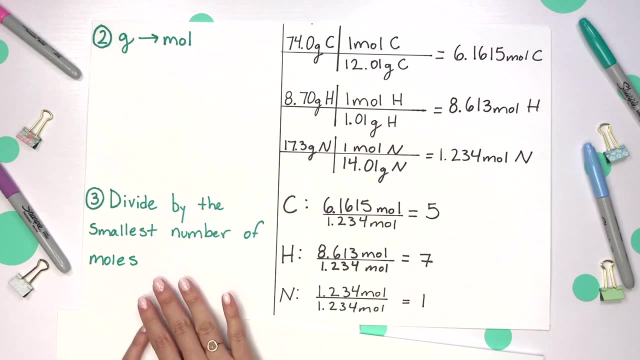 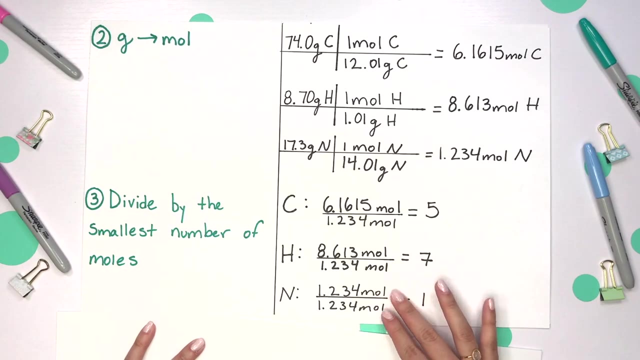 Divide these values and you get 1.234 moles of nitrogen. The next step is to then divide by the smallest number of moles, which in our case will be the nitrogen. Divide each one of these values and your moles would cancel, and we're left with the new subscripts. 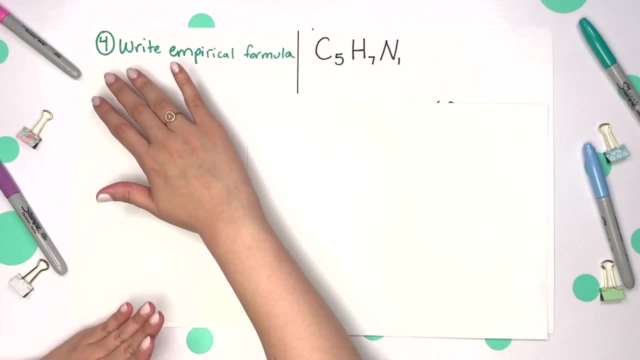 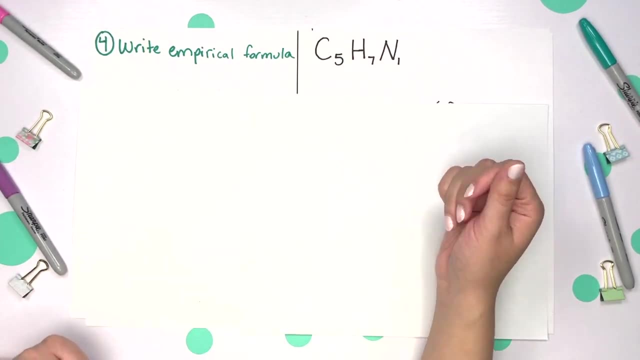 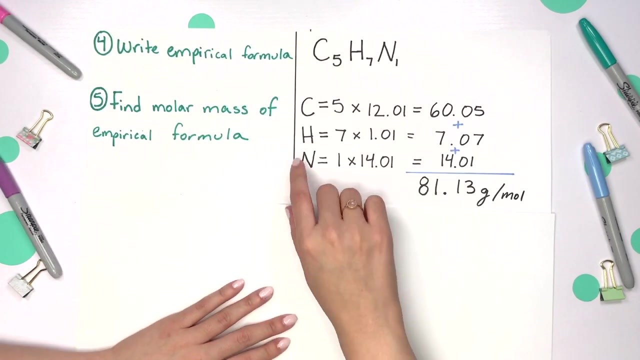 of our empirical formula. Now we have our empirical formula, Those subscripts that we found in the previous step are as shown, And now it's on to figure out our molecular formula. So the next step is to figure out the molar mass of this empirical formula. Start with your carbon, which we have five of them. 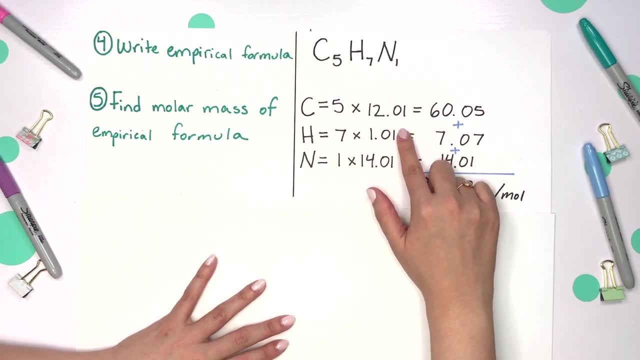 and multiply by the individual molar mass of carbon, We'll get 60.05.. Do the same for hydrogen. Now. there are seven times that, 1.01, and you get 7.07.. But there's only one: nitrogen. 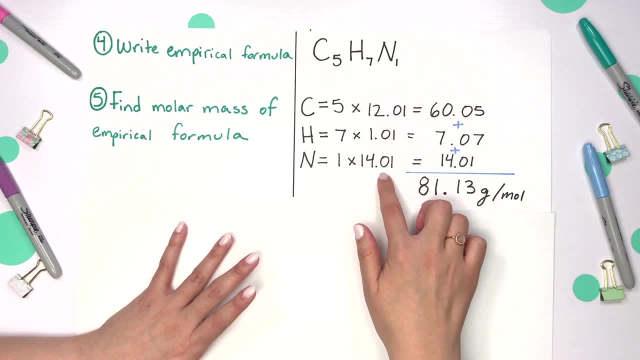 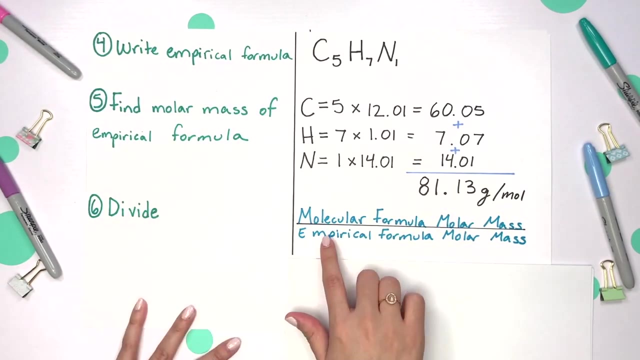 so we'll. you don't even have to really multiply. It's one times 14.05.. We'll add all these values together and your molar mass of your empirical formula gives you 81.13 grams per mole. Your next step is to divide. You will be dividing your molecular formula's molar mass divided.